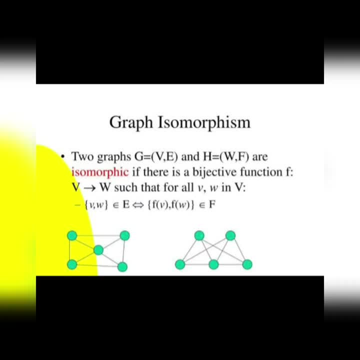 Graph isomorphism. When do we say the two graphs are isomorphic? Let's look on to the definition. Two graphs: g is equal to v, comma, a, v stands for the vertex set of g and e stands for the edge set of g. 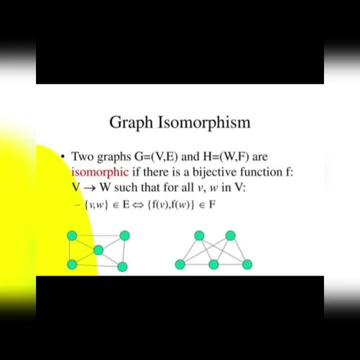 H is equal to w. comma f are isomorphic if there is a bi-jetty function, f from v to w, such that for all v comma w in v, vw is an edge of e if, and only if, f of u, f of w, is an edge of f. 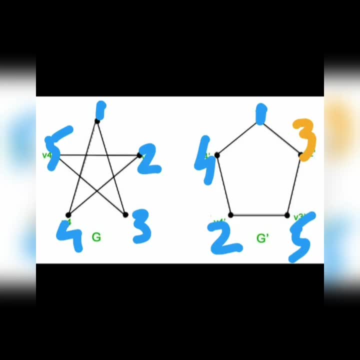 So what do you mean by that? For more clarification, let's have a look on to this figure. The vertex of two graphs is 1, 2,, 3,, 4, 5.. So similarly for g dash also, I mark all these vertexes: 1, 2,, 3,, 4, 5, etc. 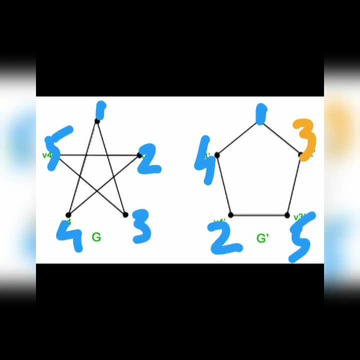 Okay. so when do we say that these two graphs are isomorphic? So if we consider any pair of edge in g, the corresponding edge must be therein, G dash. So for say, for example, let's have an edge named 1, 4.. 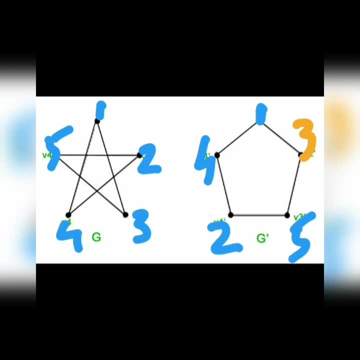 1, 4.. Just look at that edge in g: 1, 4.. Correspondingly, we have an edge 1, 4 in g dash. Similarly, 1 is incident with a 3 vertex also Okay. so 1, 3 is an edge in g. 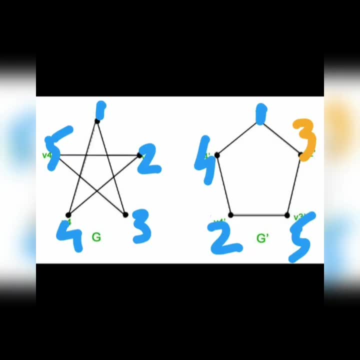 Correspondingly, in g dash also, we have an edge 1, 3.. So similarly, if any pair of u- v is an edge of g, then correspondingly f of u and f of v must be an edge in g dash. So if all these, if this condition satisfy for all the edges, then we say that these two graphs are isomorphic. 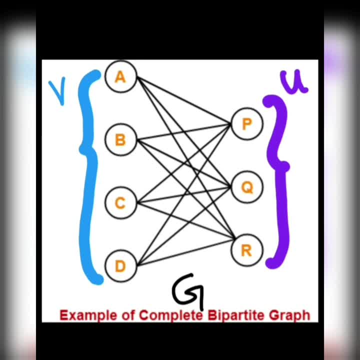 Bipartite graph. When do we say that a graph is bipartite? So let's look on to the definition. A graph g is bipartite graph if vertex set of g can be partitioned into two subsets, u and v, such that every edge of g has one end vertex in u and other end vertex in v. 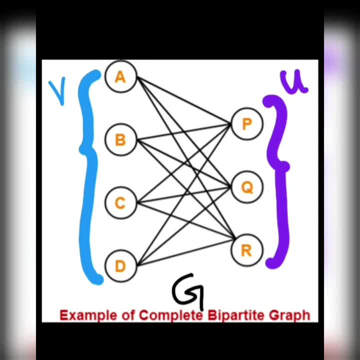 So in this graph g- let's look at this example- In this graph g I have partitioned the vertex set of G into two subsets, like u and u and v. Okay, so in the set u I have vertices like p, p, q and r. 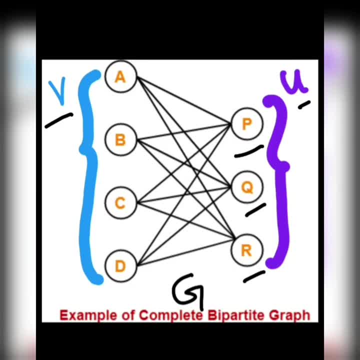 In v I have vertices like a, b, c and d. If we look at this two sets, the vertices in these two sets have one end vertex in u and other end vertex in v. But none of these vertices in U are connected to each other, but they are connected to a vertex V. 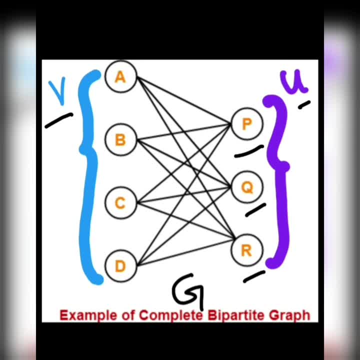 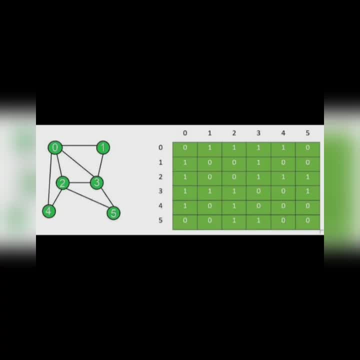 so that is what meant by a bipartite graph. Next is adjacency matrix. so what is an adjacency matrix of a graph? so, given I have given a graph, so I need to find the adjacency matrix of this graph. for that it's just like a matrix, ok, in that the rows and columns, the rows, rows. 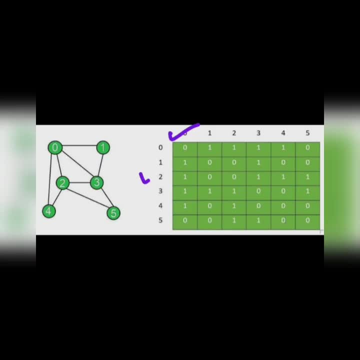 and the columns will be filled with the vertices in this graph. ok, so what will be the value inside this, inside this table? what will be the value inside this table that we are gonna find out? ok, Look at this graph Now. the vertex 0 is adjacent to 4,, 2,, 3 and 1, so if a particular vertex is adjacent to, 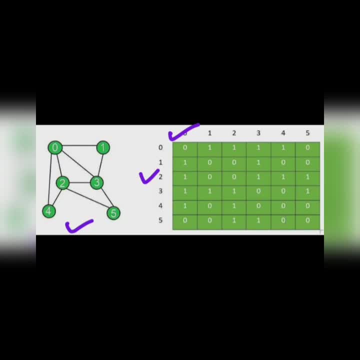 a vertex, the corresponding value will be 1. if a vertex is not adjacent with another vertex, the value will be 0. See: vertex 0 is adjacent to 1, so the value is 0.. Whereas the vertex 0 is not adjacent with the vertex 5, so the value is 0.. 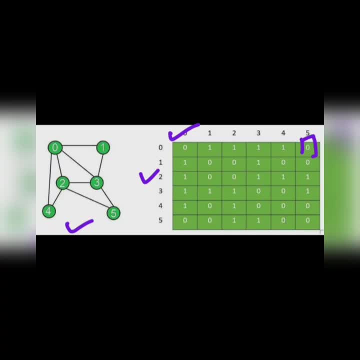 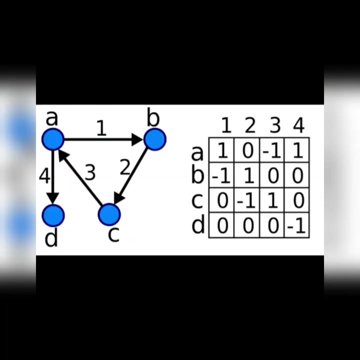 So, likewise, we will fill all the rows and columns of this matrix. so this is how we find out. this is how we find out: adjacency matrix of a graph. Thank you. Next is how to find the incident matrix of a graph. so here also, I have given a graph. 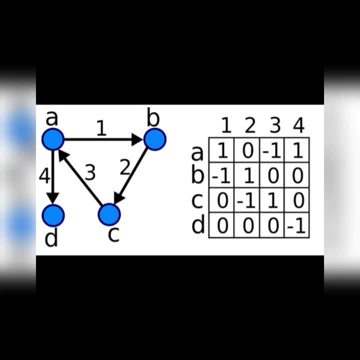 like this: I'm gonna find out the incident matrix of this graph. so here a light difference is there apart from the adjacency matrix. So here we will fill the rows of the matrix with the vertices and the column of the matrix with the adjacency matrix. I don't say area, but here we will fill the rows of the matrix. so here we will fill the. 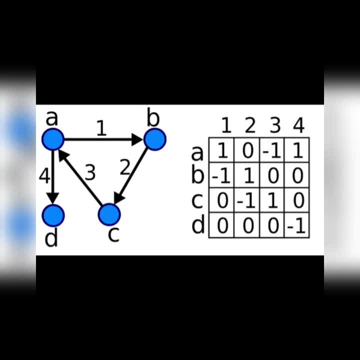 rows of the vertices. with vertices and aqui cor anterior mal ancientlüa, meaning all of our vertices, will be three individual, and that means that the address in an edge is a. Now we have put a relation value, so in which case 1 and 5.. 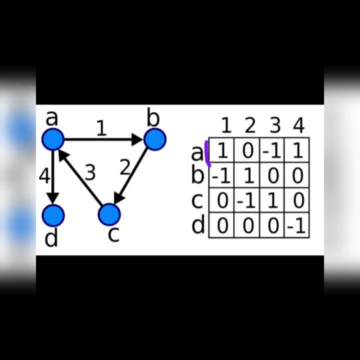 Now we are going to make a function here where we are going to say a values of the edges of the graph. ok, So if a particular vertex is adjacent to an edge, there value will be 1, here the vertex 2, so the value is 0. so likewise, we will fill all these values in the table. so this is how we find. 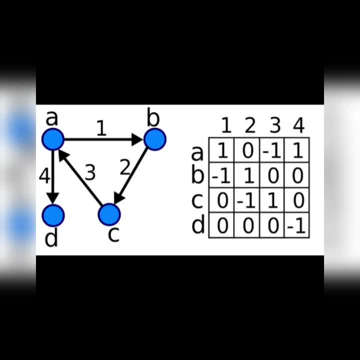 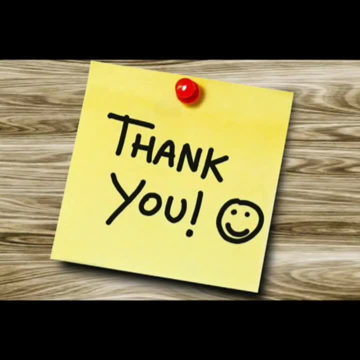 out the incident matrix of a graph. so this is all about this video. if you like my video, do not forget to like, share and subscribe to this channel, thank you.